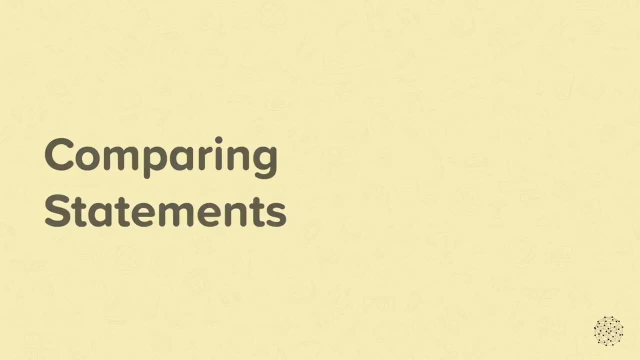 Comparing statements. Charlie the crocodile is very greedy and always wants to eat the larger value. This means the left hand side is less than the right hand side, and we use this symbol to show that. This means the left hand side is more than the right hand side, and we use this symbol to show that. 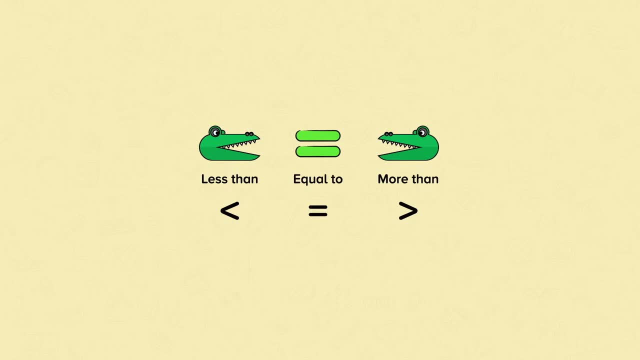 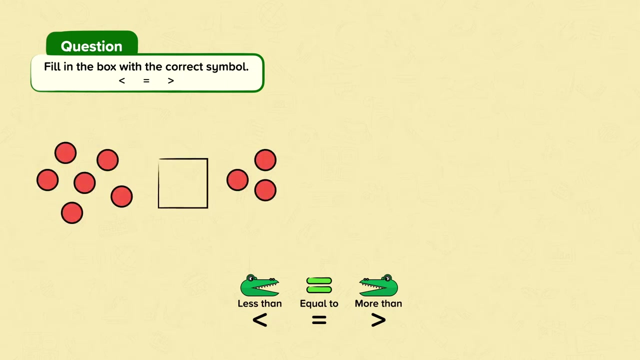 This symbol means both sides are equal. Fill in the box with the correct symbol. Here are the symbols to help us: Which side is more. Here we have six dots and here we have three dots. Which side will Charlie the crocodile want to eat? 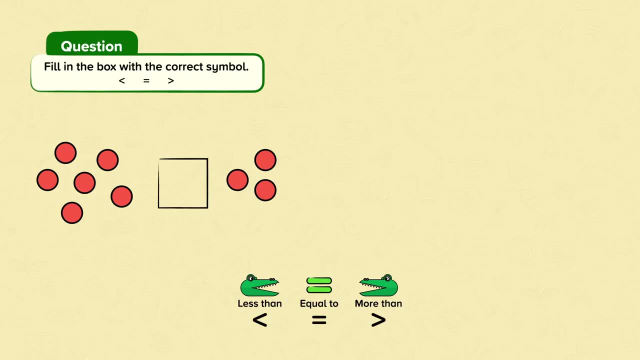 Which side is bigger? We need to use this symbol. We know that six is more than three. Now it's your turn. Which symbol goes in this box? Charlie the crocodile will eat the larger side. We know we need to use this symbol. 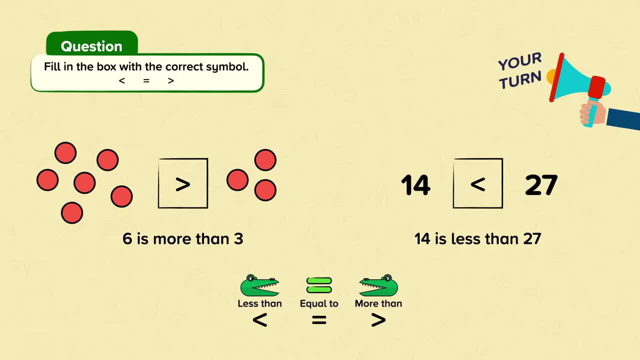 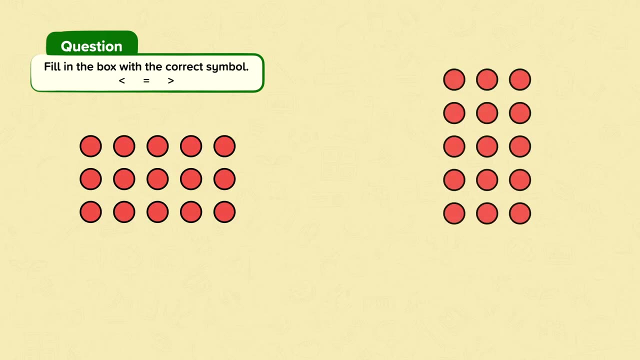 Fourteen is less than twenty-seven. Well done. if you got that correct, Fill in the box with the correct symbol. We need to compare these two number arrays. This group shows three rows of five or three groups of five. This is the same as three times five. 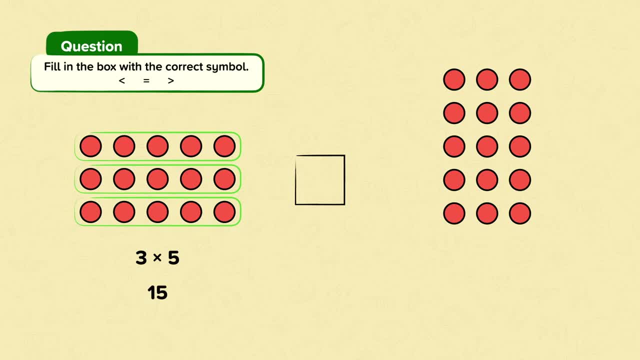 which is fifteen. This group shows five rows of three Or five groups of three. This is the same as five times three, which is fifteen. Which symbol do we need to put in the box? We need to put in this symbol? We know both sides are equal. 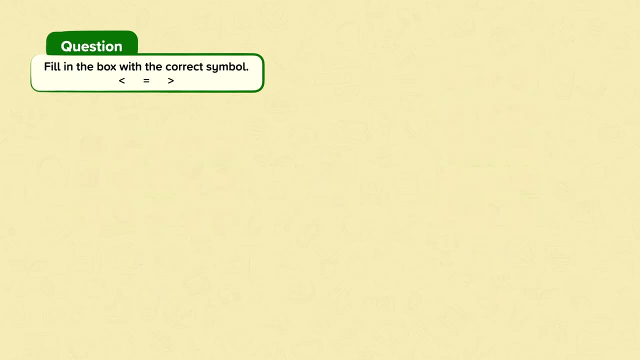 Fill in the box with the correct symbol. We need to compare these two number arrays. This group shows four times four. We have four rows of four or four groups of four, which is sixteen. The second group shows five rows of three or five groups of three. 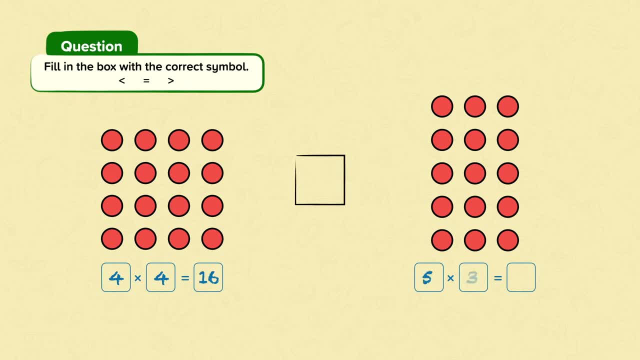 This is the same as five times three, which is fifteen. Remember, Charlie the crocodile is very greedy and wants to eat the larger side. Which side will Charlie the crocodile want to eat? Which side is bigger? Sixteen is bigger than fifteen. 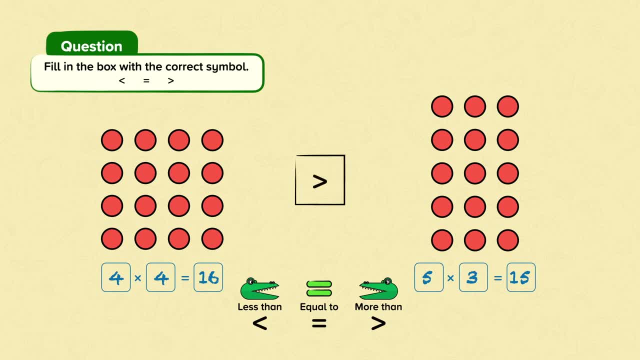 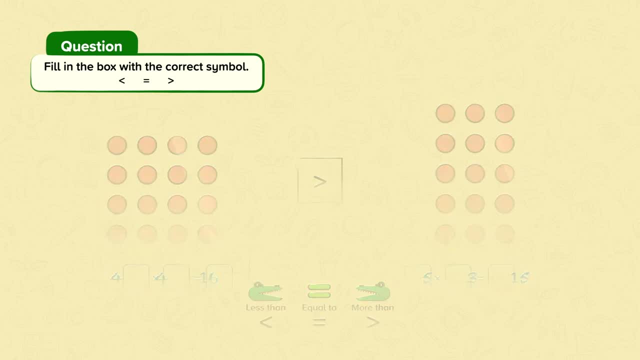 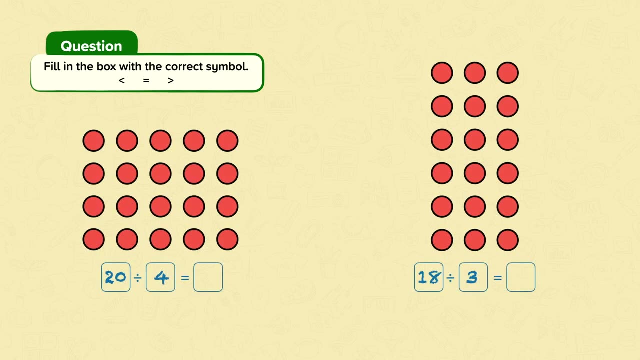 so we use this symbol. We know that four times four is more than five times three. Fill in the box with the correct symbol. We need to compare these two number arrays and use them to help us with our division. Twenty divided into four equal groups. 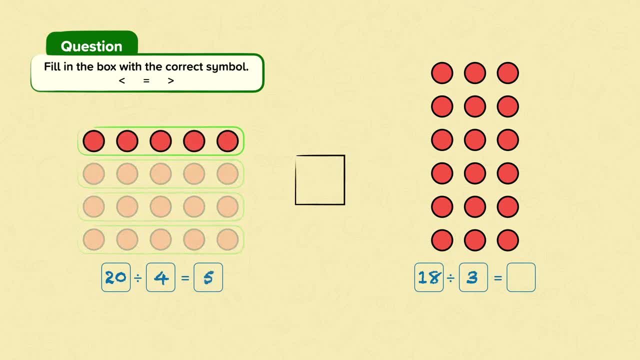 equals five. Eighteen divided into three equal groups equals six. Which side is larger? Which side will greedy Charlie the crocodile want to eat? Charlie will want to eat this side. Twenty divided by four is less than eighteen divided by three. Fill in the box with the missing number. 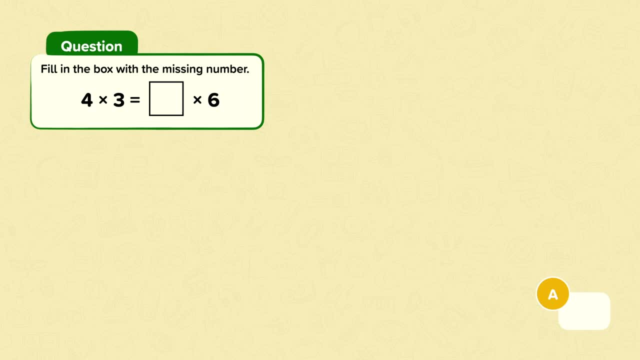 First, we know both sides of this equation must be equal to each other. We can use this number array to help find four times three, Four groups of three, or four times three equals twelve. So we know twelve equals something times six.